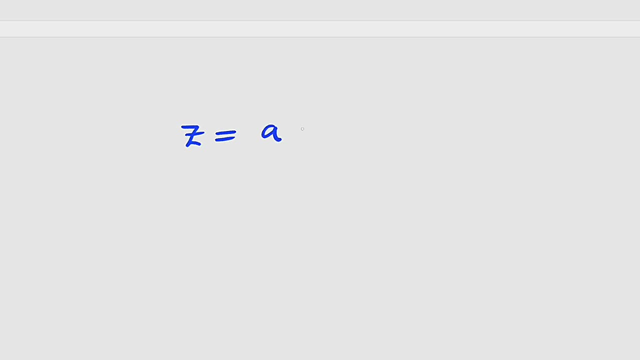 a complex number, z, given as a plus b- i, The real part which is donated by Re of z is equal to a, while the imaginary part of this complex number z is just the coefficient of i- b. So this is what we are going to learn, how to do, and if we are given this and this, we'll be able to form a complex 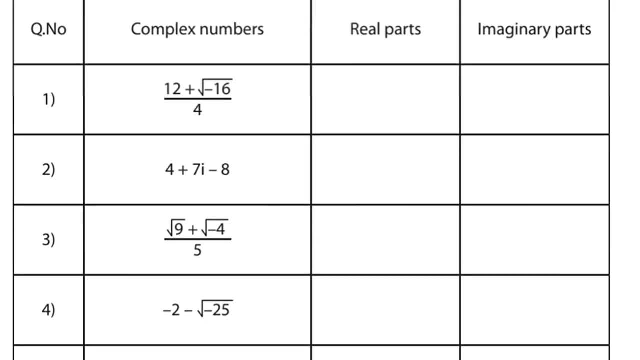 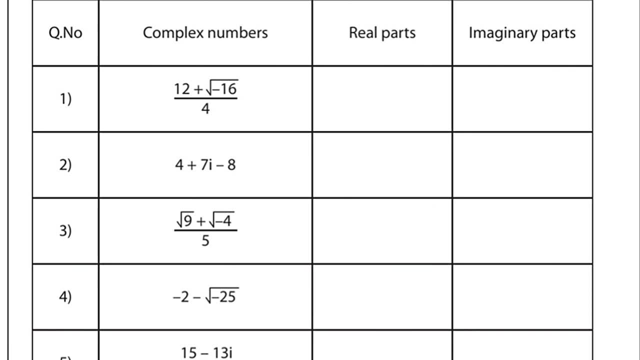 number. All right, let's get started. So the first one we are given 12, plus the square root of negative 16 divided by 4.. I want you to know that the real part is only 12 divided by 4, because you know. 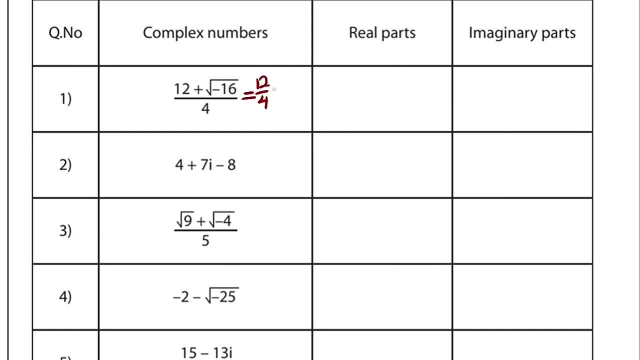 we can split this as 12 divided by 4, then, plus the square root of negative, 16, also divided by 4.. So the real part is just 12 divided by 4, which I can write as the real part of z equal to 12 divided by 4, which is equal to 3.. 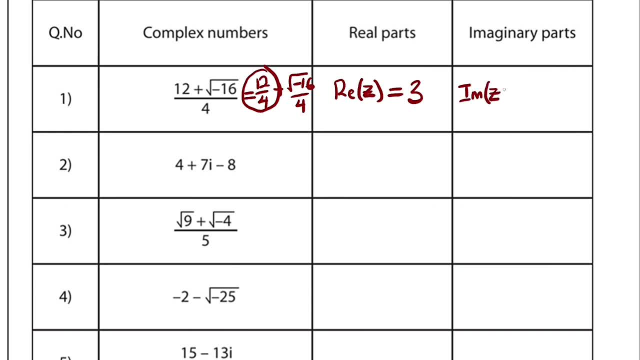 What about the imaginary part of this z? The imaginary part will be the square root of negative 16 divided by 4.. Square root of negative 16, remember, is 4i, right, but 4i divided by 4, because we have four here, will give us i, But the imaginary part is just the coefficient of i, So the 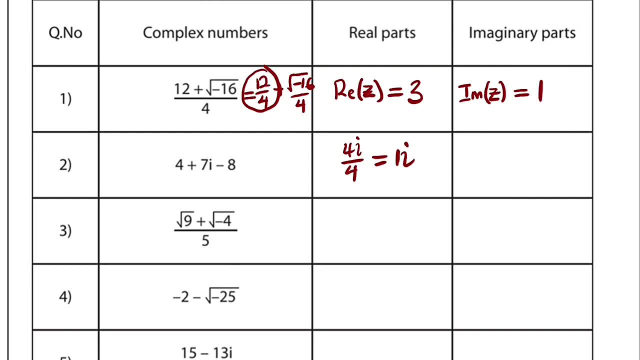 coefficient of i here is 1, so we have this as 1. the second question: we have 4 plus 7, i minus 8. you know we can rearrange this equation as 4 minus 8. then plus 7 i, 4 minus 8 is just the real part. 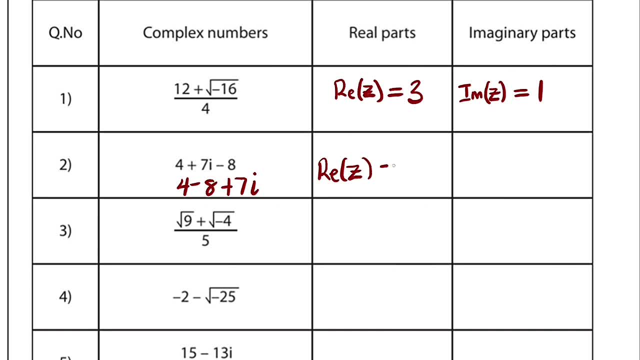 so we have the real part as what negative 4, because 4 minus 8 is negative 4. but what about the imaginary part? is going to be 7, the coefficient of i question number three. we have square root of 9 plus square root of negative 4, all divided by 5.. the real part will be square 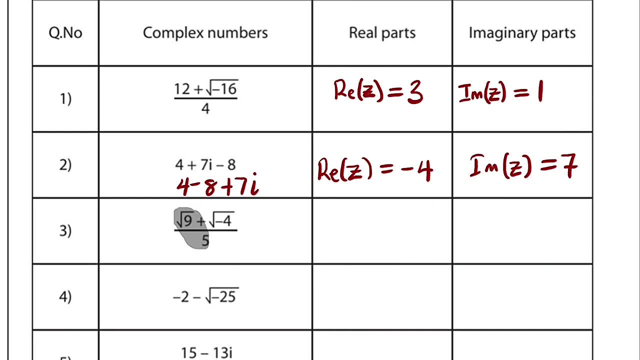 root of 9 divided by 5. and square root of 9 is equal to 3 divided by 5. therefore, the real part of this complex number is equal to 3 divided by 5.. moving on to the other side, we have square root of negative 4 divided by 5. square root of negative 4, remember, is 2: i and we have 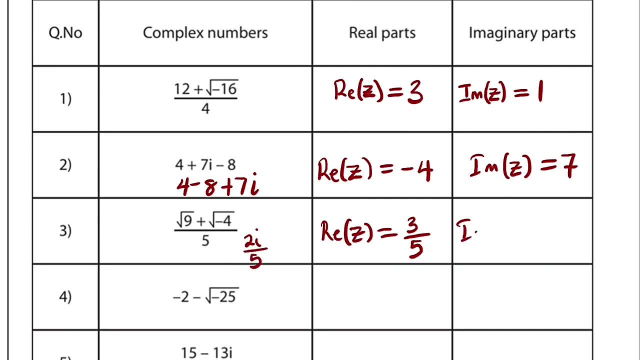 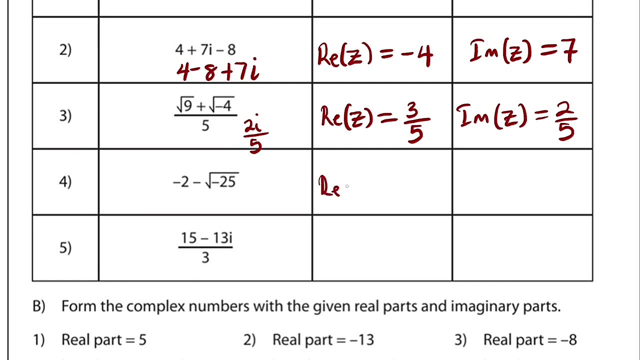 to divide it by 5, which implies that the imaginary part, which is just the coefficient, is 2 divided by 5.. moving on to question number 4, the real part is clearly written as negative 2, so we have the real part as negative 2.. while the imaginary part is: 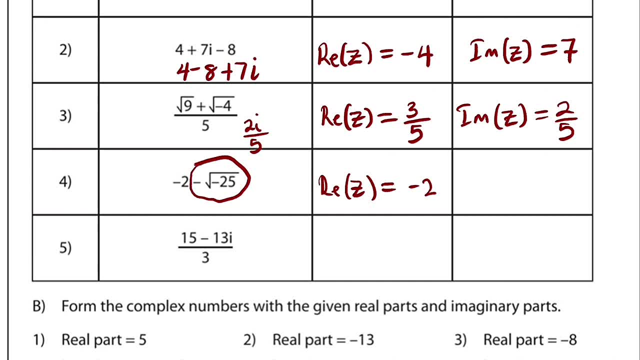 negative. you have to include this negative negative. the square root of negative 25, square root of negative 25 is 5: i. but we have a negative sign, so we have negative 5 i. so what is the coefficient? negative 5? therefore, the imaginary part of this complex number is equal to negative. 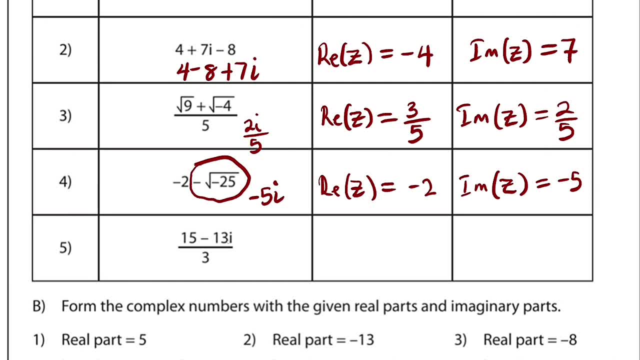 5. question number 5: 15 minus 13 i divided by 3, the real part will be 15 divided by 3, 15 divided by 3, and the imaginary part will be negative 13 divided by 3.. the imaginary part is equal to negative 13 divided by 3 and we are done with this part. 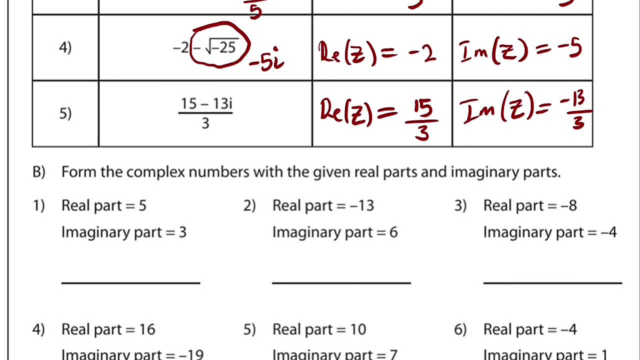 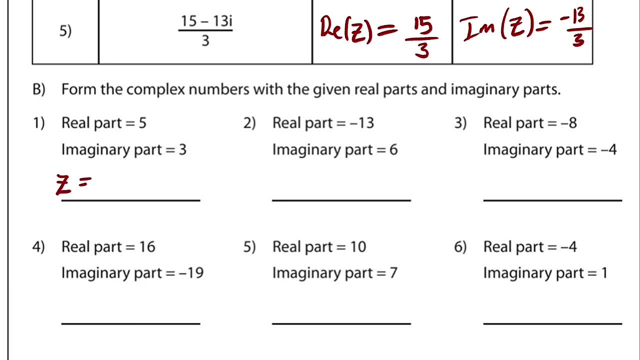 what about the second part? we are given the real and imaginary parts and we want to form the puzzle, to form a complex number at that point. so the complex number here is equal to the real part, which is 5. then plus the imaginary part, which is 3, 3, then you bring your i. 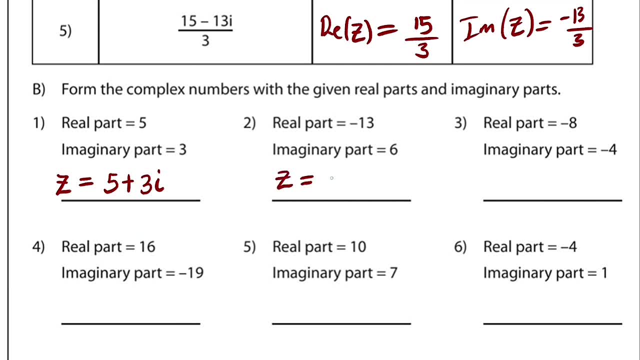 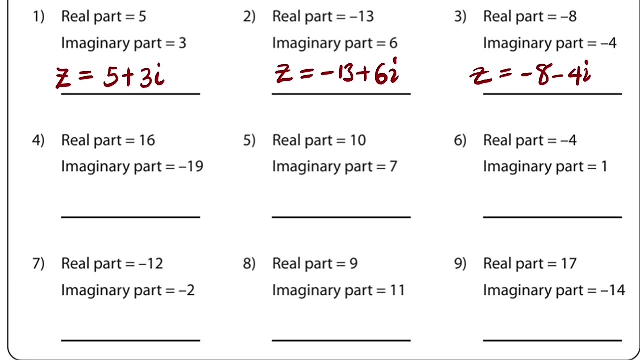 coming here, we have negative 13 as the real part. negative 13 plus the imaginary part 6, i number 3, z equal to negative 8. then minus 4i number four. they are as simple as that. so let me do four, five, six and leave the rest.